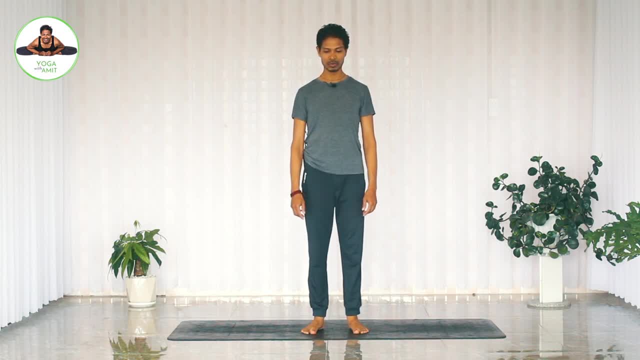 and take moments to come onto the mat, into the present moment. once you're ready, roll your shoulders up, back and down a few times and then other side back up forward. good, then take your right hand, stretch the hand and bring to the side and then take the. 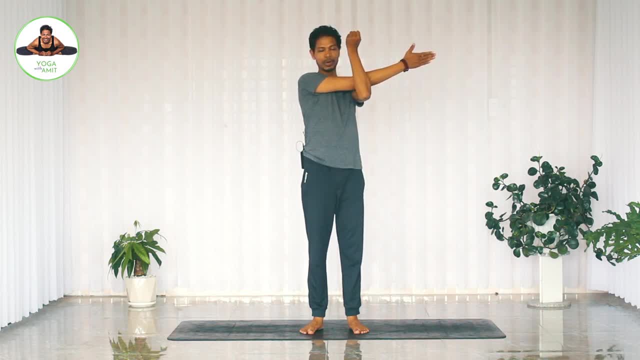 another hand and interlock and then try to press it inward out. do what is comfortable and press as much is easier in your body. good, chain the side left arm. let's do that three times, gently push, gentle push and see what feels best. good, then bring your hands onto your shoulders and 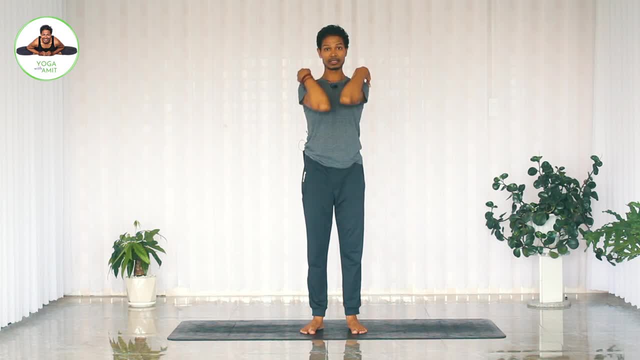 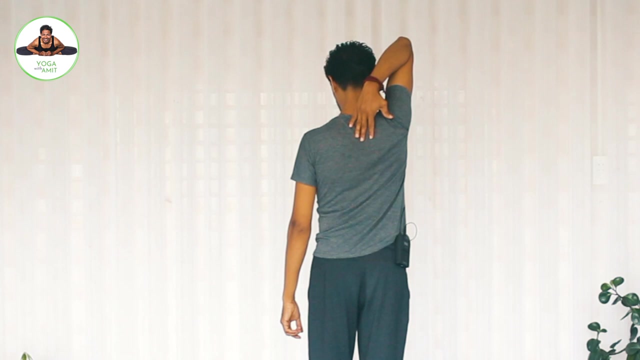 rotate your shoulders as wide circle as is possible in your shoulders. it depends on the mobility of your shoulder joints to be able to rotate wide, so do what is exactly possible in your body other way around. good release. then bring your right arm up like this: then take the help of your left. 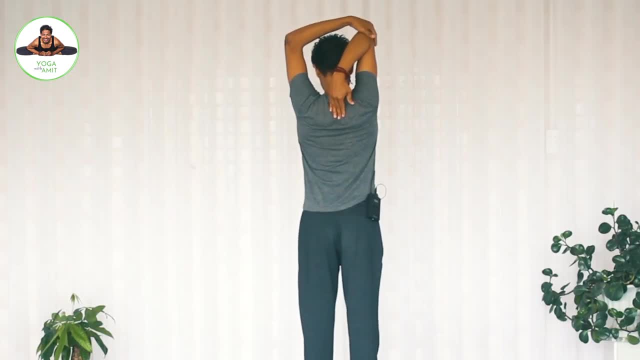 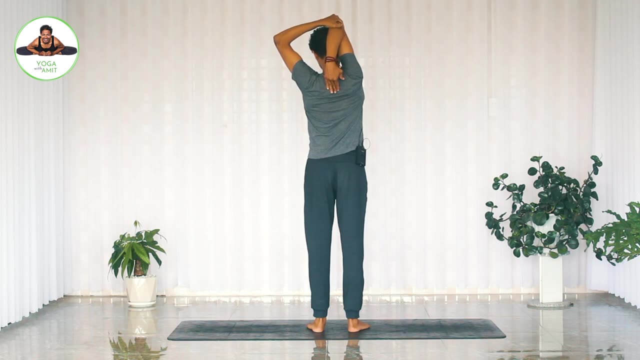 arm to pull the shoulder or the elbow slightly inward. release chain the hand, so left hand goes basically it's in the middle of the shoulder blades and hold with your hand and push gently, release. let's do that also three times, release forth. this is a starting của. 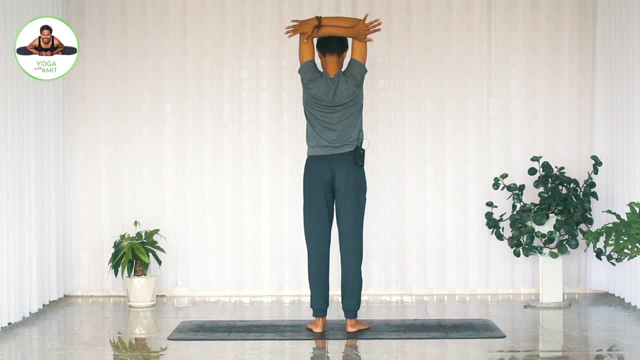 good, then interlock your both elbows like this, so holding your elbows, inhale as you exhale, bend to the right like Inhale back, exhale to the left, Inhale back, exhale to the right, Inhale back, exhale to the left. 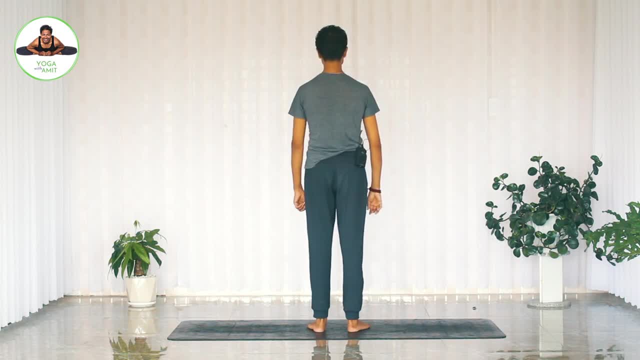 Inhale back and release. Release the tension from the shoulder once and then interlock your shoulders and elbows again like this: Now inhale As you exhale, twist to the right, Inhale back, exhale to the left. 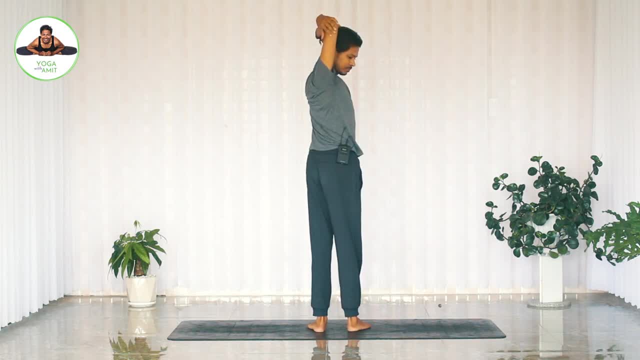 Inhale back exhale to the right. Inhale Inhale back exhale to the left. Inhale back exhale to the right. Inhale back exhale to the left, Back to the center and release. 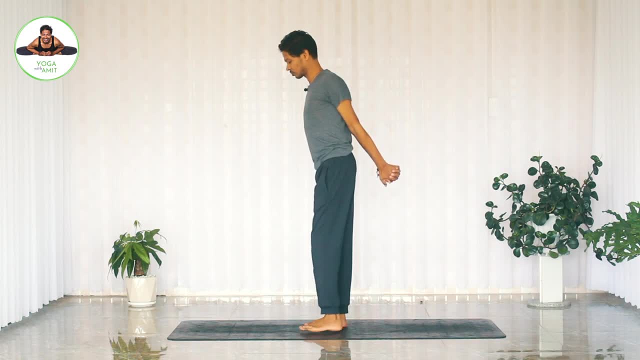 Then interlock your hands on the back Feet about hip width apart. Inhale, Inhale, Exhale. push your hands towards the ground, Inhale back. Let's do that 5 times. Inhale. 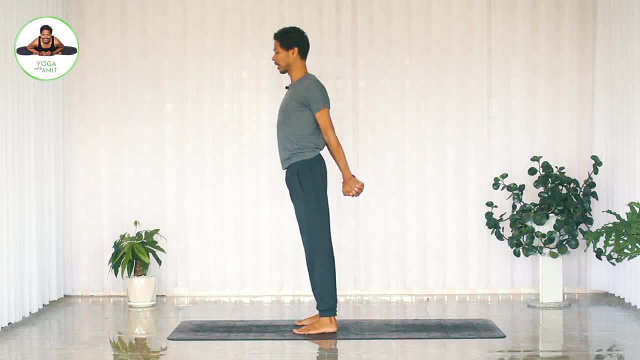 Exhale. Inhale back. Inhale Exhale. Inhale back. Exhale Inhale. Exhale. Inhale back. exhale. inhale. exhale down. come back last round. inhale exhale come. 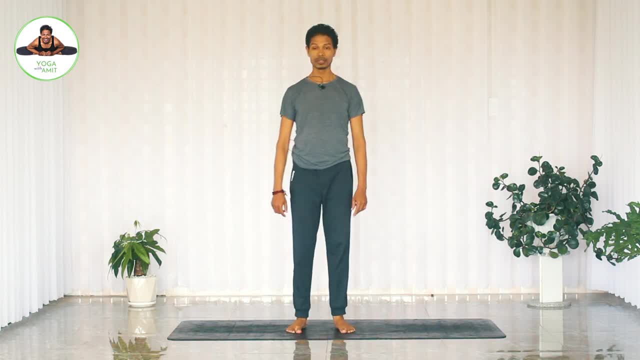 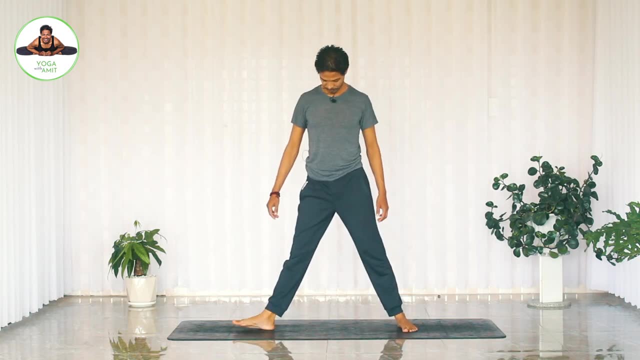 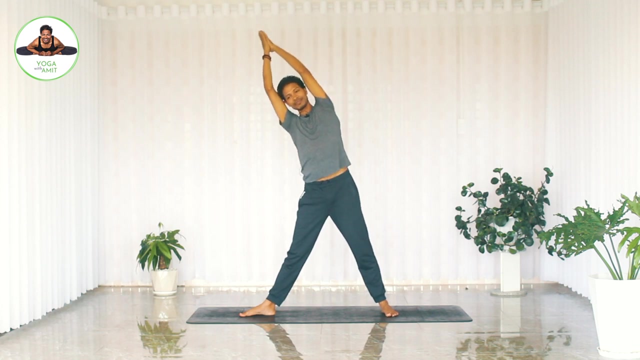 back and release. Rotate your shoulders, let go the tension. then open your legs. take your right foot out, palm together- inhale as you exhale. bend to the right- inhale back. exhale to the left- inhale back. exhale to the right- inhale back. 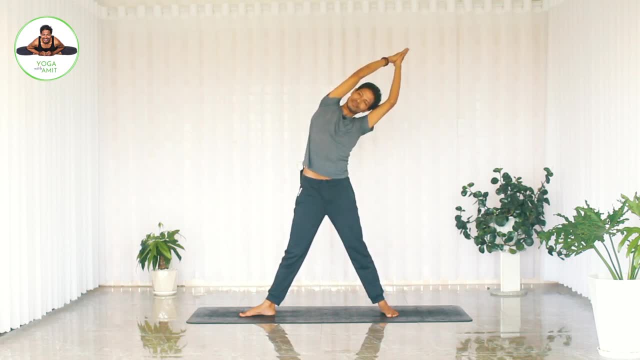 exhale to the left, Back to the center. change the leg, right foot in, left foot out. inhale as you exhale. bend to the left, inhale back. exhale to the right, inhale back. exhale to the left inhale. 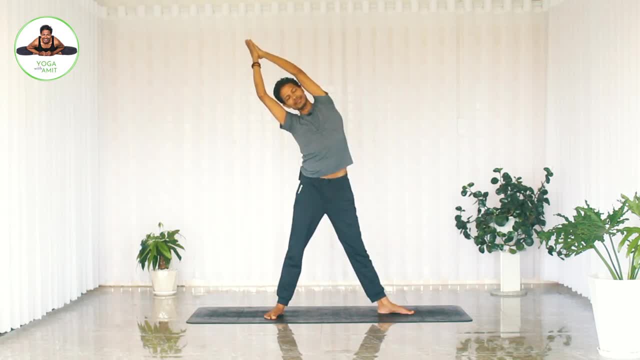 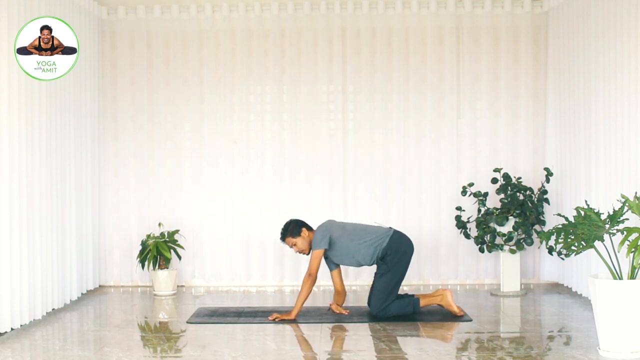 back. exhale to the right. Exhale. take your left hand straight as you exhale. Come back and let's go into the cat pose bhajania radhyacchana inhale. bring your right arm up. exhale. bring your right hand under the left thread, the needle side of the head. он the 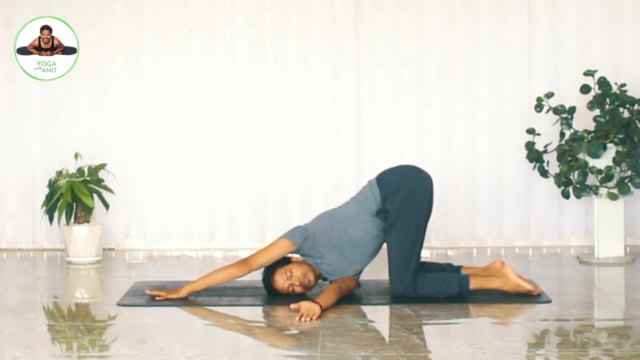 ground. extend your left arm out, Exhale. bring your right hand under the left. thread the needle inside of the head on the ground. Windmill to bhajana: Out 0. Then, once you are comfortable, inhale, bring your right arm up and exhale. bring it back. 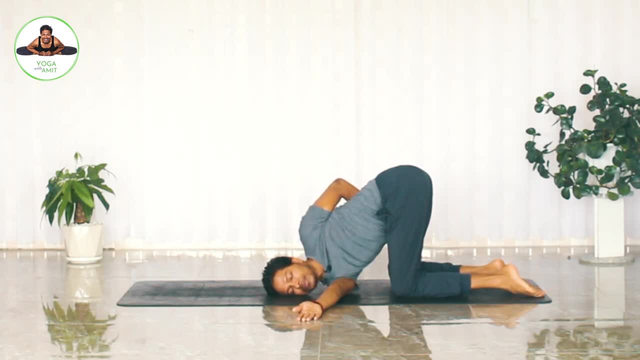 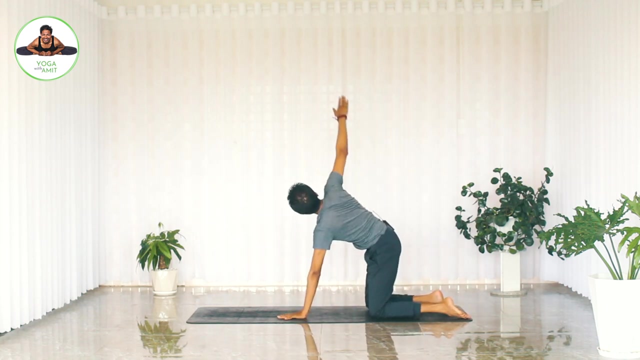 onto your back- Inhale, back- exhale. bring your hand down. push with your hand and bring the right hand back towards the ceiling. Exhale, release. change the left hand. inhale- left arm up- Exhale. bring the left hand under the right temple on the ground side of the forehead. 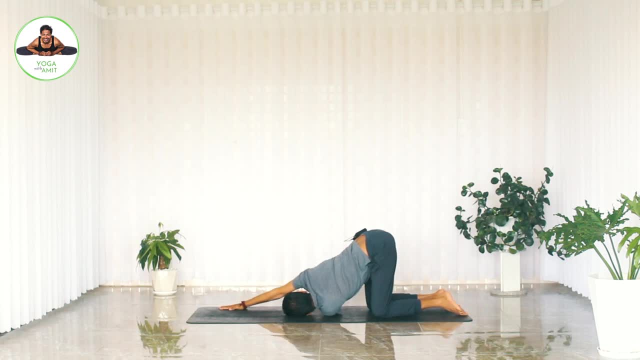 on the ground, Extending the right arm out. once you are ready, inhale- right arm up, exhale. bring the right hand onto the back or hold your thigh if possible. Inhale, bring your right arm up, Exhale- release. push with your hand. bring your left arm towards the sky or ceiling. 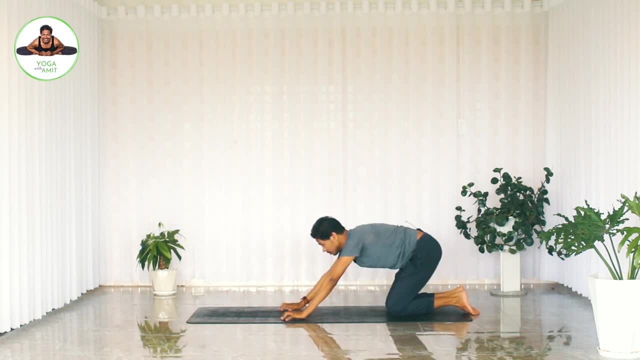 Exhale down and lay onto your belly, Forehead onto the ground. Check your hands under your shoulders, Inhale, Inhale, push with your hands, lift your chest up, relax your shoulders and tuck your elbows by the side. look forward or up. 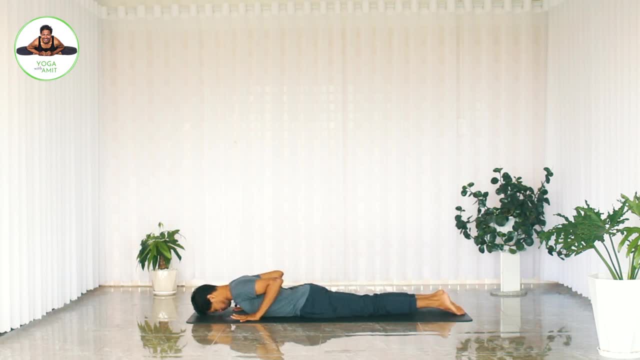 Exhale down. Let's repeat that three times: Inhale up, Exhale down. Inhale up, Exhale down. This time we are going to do side cobra Push with your hands, inhale.